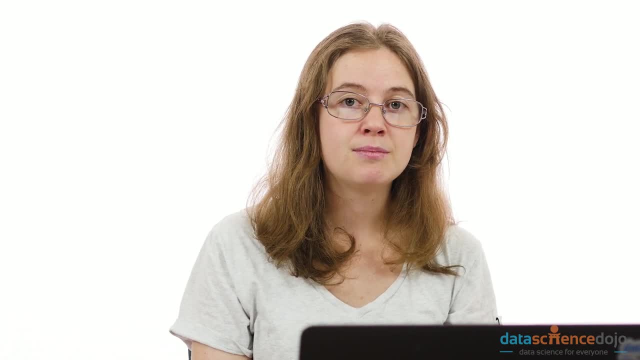 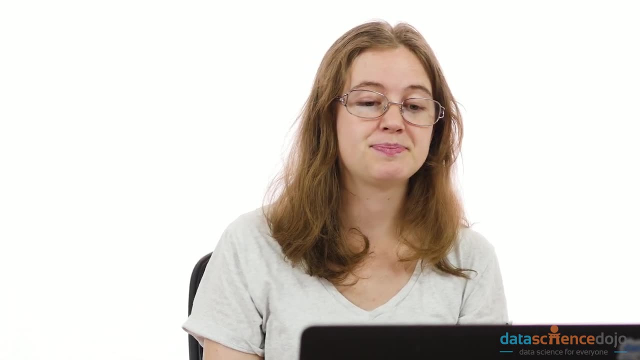 manually tell R the data type for every single column. But it's really important to know your main data types so you can check what kind of values you're working with when modeling data or when casting it as a certain data type. So let's first look at your numeric types or numbers. 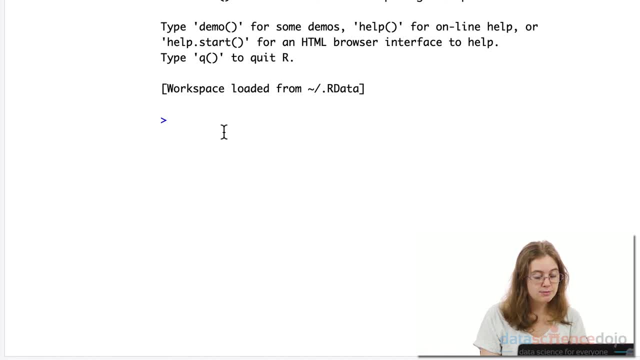 that measure things in your data. So you can get a whole number or an integer. You can get a number with a fraction or a floating point number. A floating point can be more than one number, before or after the decimal point. Something to note when printing the result of a floating point. 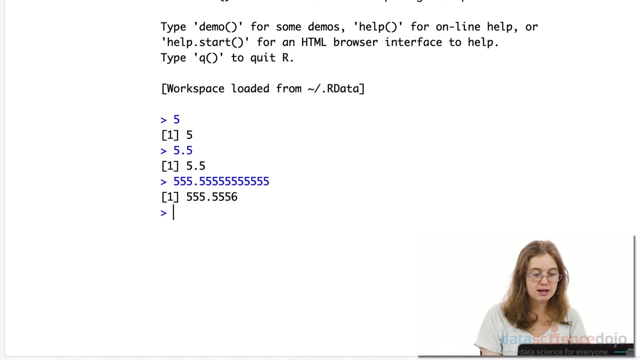 number R usually rounds this up to five places after the decimal point, so it won't just print, you know, an infinitely long set of numbers after the decimal point. You can also print a number with a fraction or a number after the decimal point. 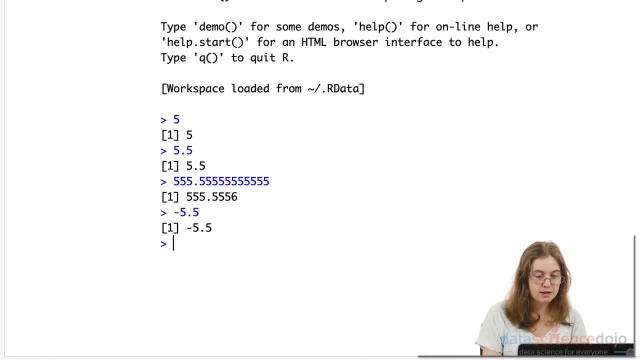 You can also have negative numbers, And so the same basically applies. So R classes all these kinds of numbers as one data type called numeric. So if you use the class function here and you give it any of the numbers that we've mentioned, you'll see that it's classed it as numeric. 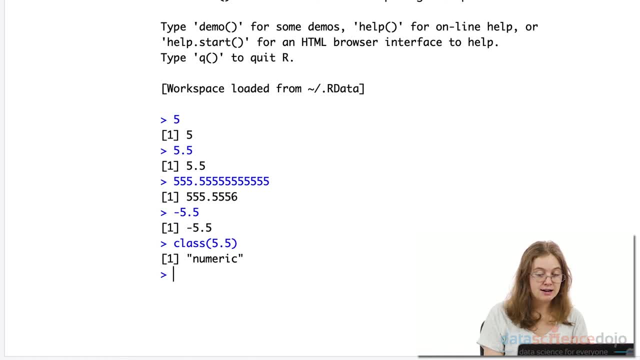 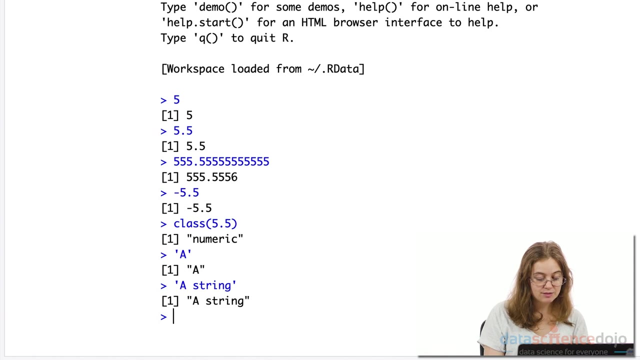 Another common data type you're going to often see in many datasets is character. So this could be a single character or it could be a string of characters. It could also be a number represented as a string. All these are classed as character in R, So if we use the class function again, 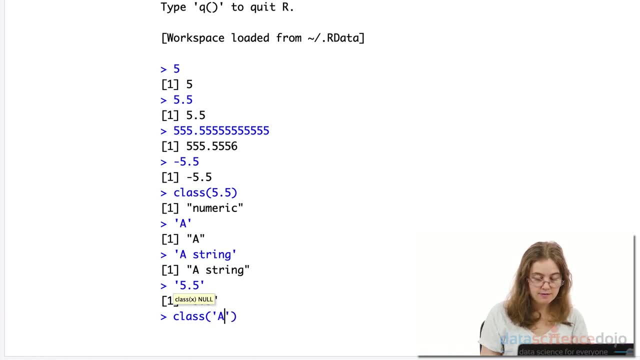 and we give it any of the string characters, you'll see that it classed it as character. You can also use double quotation marks so that words with apostrophes are not incorrectly interpreted as single marks around a string. So, for example, won't using an apostrophe. 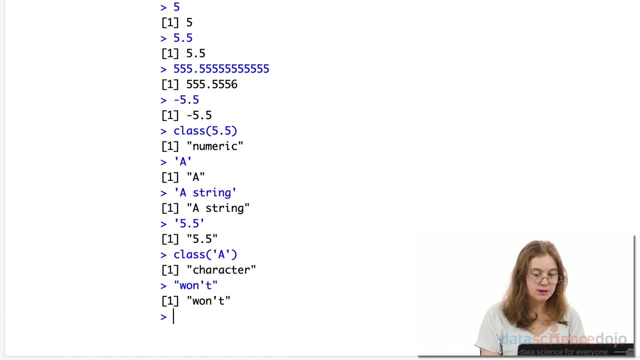 Another way you can write this is to use the escape backslash to read it as a little apostrophe and not a quotation mark around a string. So, for example, won't using an apostrophe to read it as a little apostrophe. So the data type character can be used for text strings or unique names of things. 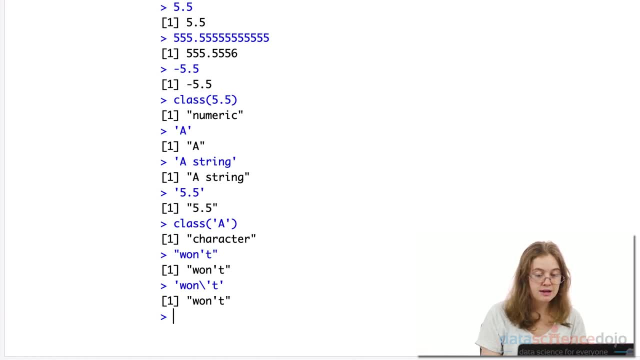 Otherwise they can be casted as factor levels or categories. Later in the video series we'll discuss the R object. factor Logical or Boolean data types are also common, So where there's kind of a true or false value, so the presence of something or not. So for example, a variable on benign cancer might show 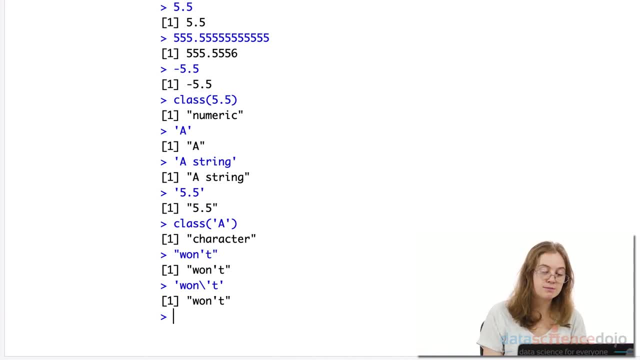 its values, as some people to be true in having these cancer and some people- some people- to be false- in not having this cancer. So if we import true or false into our class function here, you'll see that it probably classes it as a logical data type. 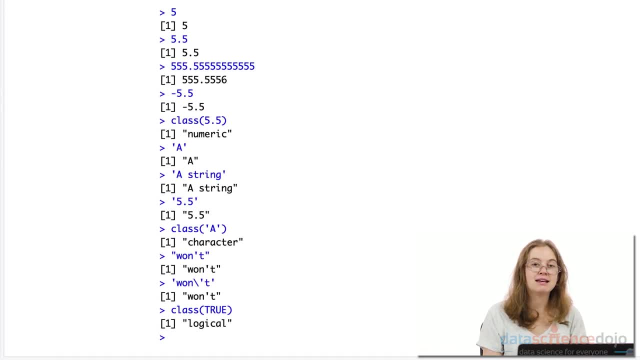 And that's it. You now have an understanding of the main data types you're likely to get in your data sets. The next video we're going to cover variables. 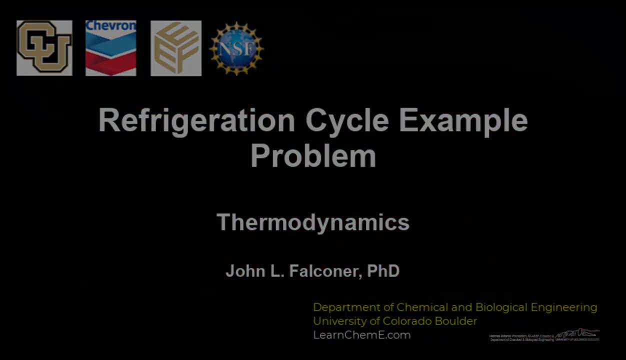 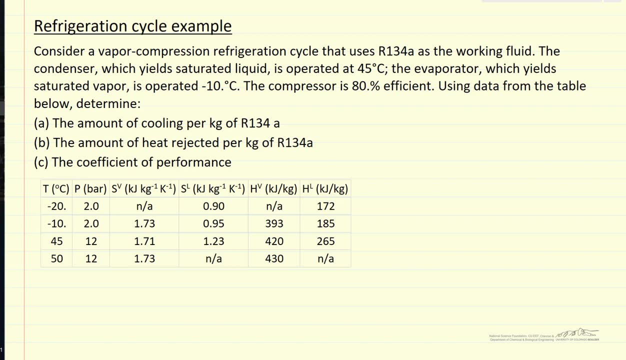 In this example, we're going to work through calculations for a vapor compression refrigeration cycle And, to make it easier to follow, we've put the data that we're going to need into a table to avoid having to search through tables to understand what's happening And 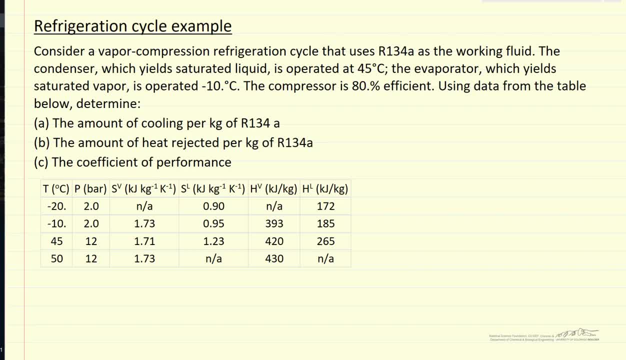 best way to look at the information is to look at a pressure enthalpy diagram. that tends to be most useful for refrigeration, So we're going to put the data given in the problem statement into this diagram, where the phase envelope looks something like this: And now 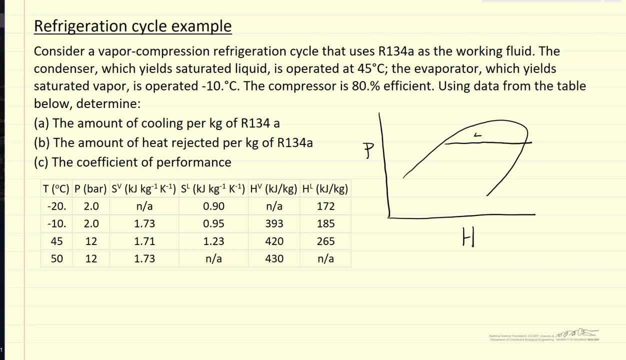 the problem states that the upper pressure corresponds to a temperature of 45 degrees C. It says we reach saturated liquid here. The course going through the throttle is at constant enthalpy, And then the lower temperature is minus 10 degrees. so this is minus 10 degrees.